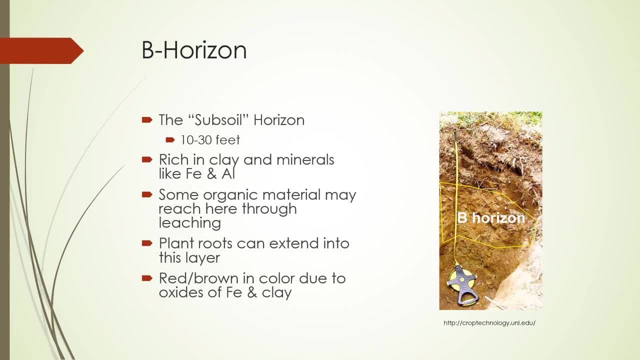 It's very rich in clay and minerals Such as iron and aluminum. You may get some organic material that reaches here through leaching. some plant roots may be down there and If you've got red and brown color, that's due to oxides of iron and clay and that would be a well oxygenated soil. 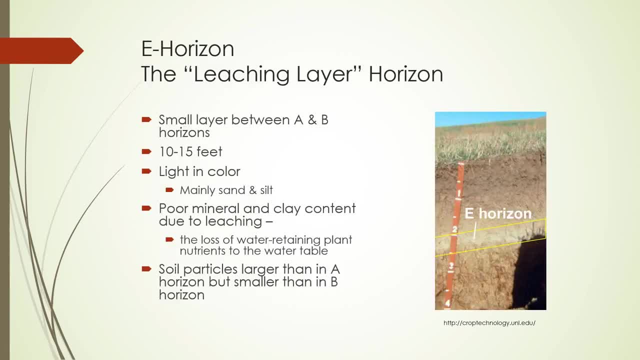 Not very common in our particular area. Okay, the e horizon is called the leaching layer and that's the small layer between a and B. It's 10 to 15 feet deep, very light in color and It's going to be mostly sand and silt. 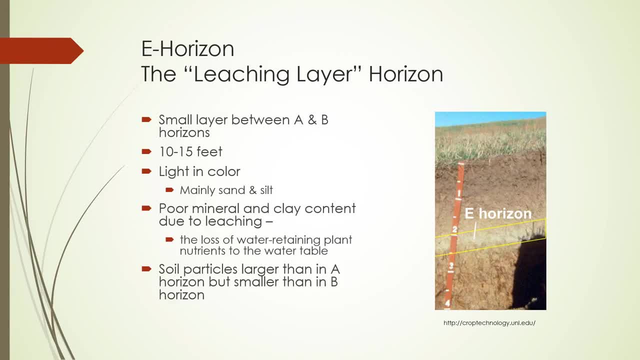 doesn't have a lot of mineral and clay content because it's leached, and This is also where water retaining plant nutrients are leached into the water table. Soil particles that are here are larger than in the a horizon but smaller than in the B horizon. 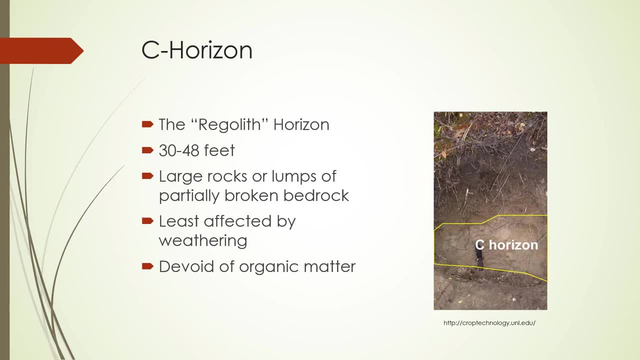 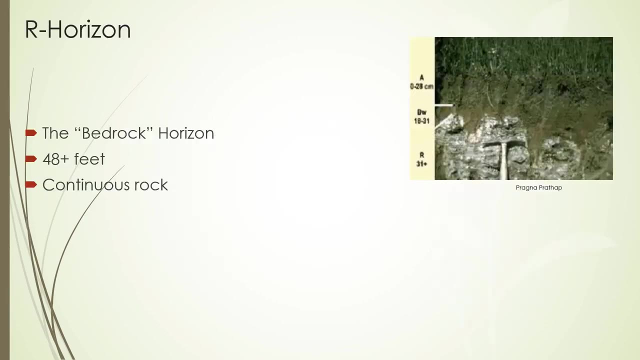 Okay, so the sea horizon is the regolith horizon or rock horizon: 30 to 48 feet deep, large rocks or lumps of partially broken bedrock. it's the least affected by weathering and you're not going to find any organic matter in this area. and then, finally, we have the our horizon, which is 48 feet and deeper. 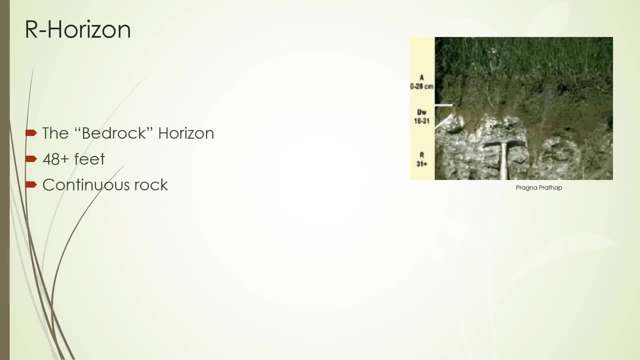 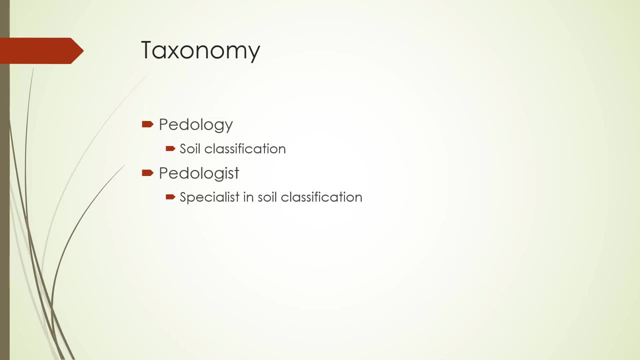 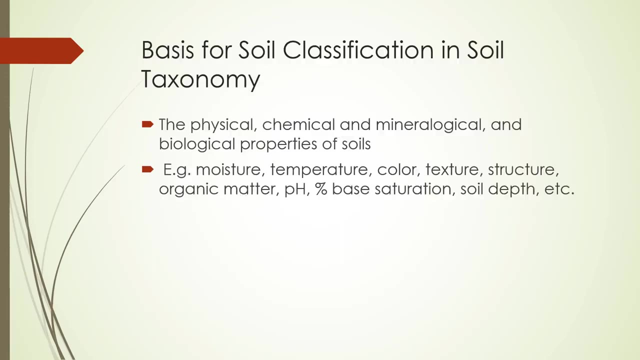 and it's continuous rock and that just depends on what your parent material is as far as what type of rock you might find here. okay, so podology is the study of soil classification and a podologist is a special in soil, specialist in soil classification. so soil classification is based on the physical, chemical and 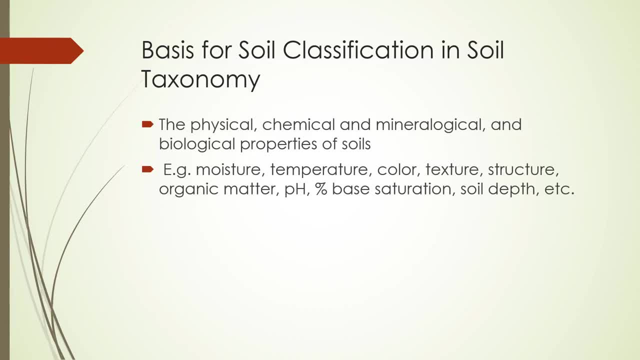 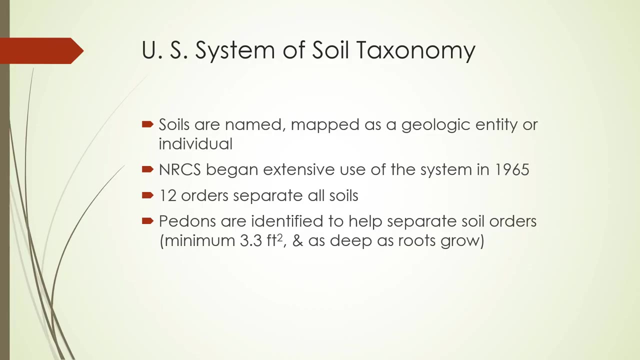 mineralogical as well as biological properties of soil, and some of the traits may also contain moisture, temperature, color, texture, structure, organic matter, pH, soil depth, etc. so soils are named mapped as a geologic entity or individual, and the NRCS, which is the Natural Resource Conservation Service. 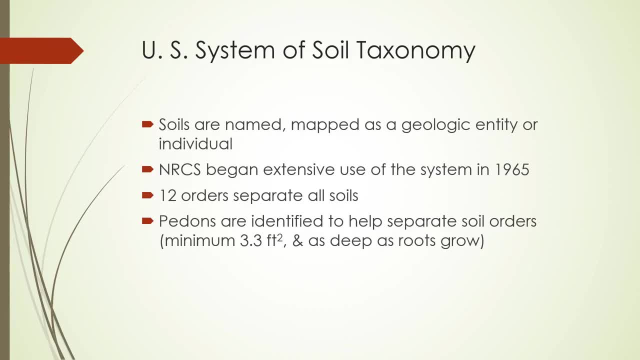 began use of the system in 1965 and there are 12 orders that separate all soils, and some areas may actually have all 12 soil types. believe it or not, Hawaii has all 12 soil types, so this might be fairly easy to follow up with if you're Jim. 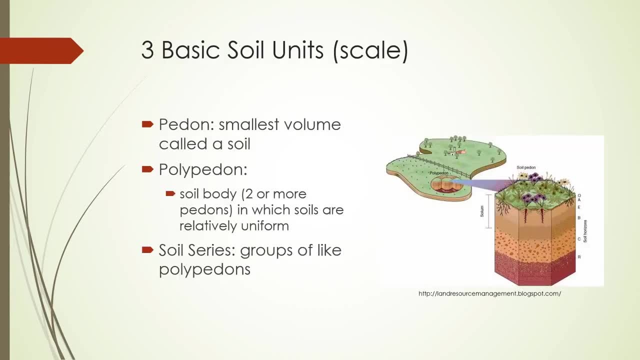 and some of the related species of soil, from this onそんな're um, and hopefully you can find more ссылas in my other book that talks about this. shouldn't forget a arson: the America. küंüç置u. yeah, all, of course, as we looked between eating. 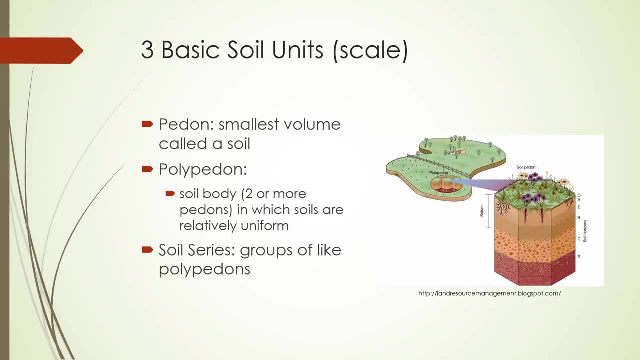 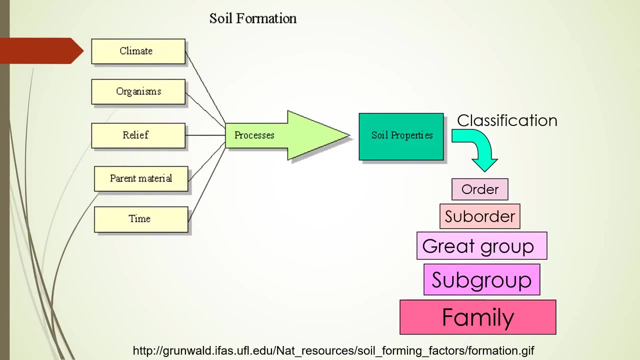 i'm going to go ahead and start with our soil as Motor. Maddie Mur pic's the bioạnalysis for our soil as well. if you go through the formula of MCD, there's a. this is soil formation. you've got your climate or organisms relief parent. 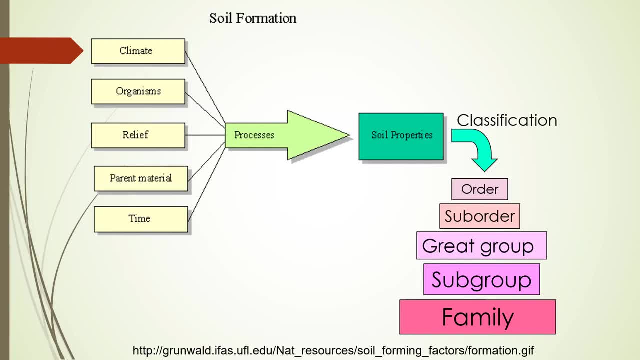 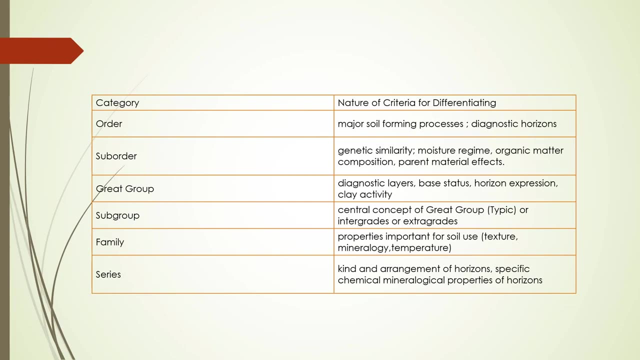 material and time. then there are processes that happen and then the soil properties help with the classification. and while there are a lot of different tiers to this, we are primarily looking at order and family. so in order are major soil forming processes, this is diagnostic horizons, family, our property. 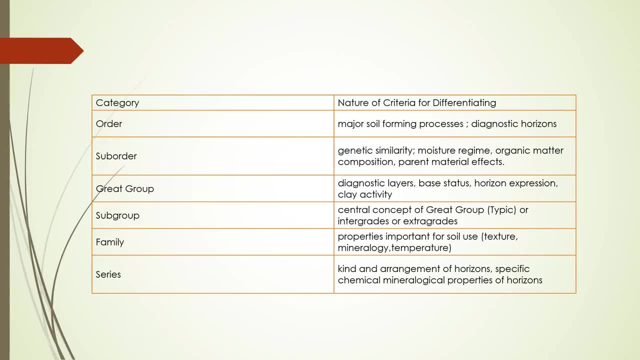 is important for soil use, such as texture, mineralogy and temperature, and series is the other one that we're looking at and that's kind and arrangement of horizon, specific chemical mineralogy, mineralogical properties of horizons. we'll talk a little more about that in a minute. okay, so when you're 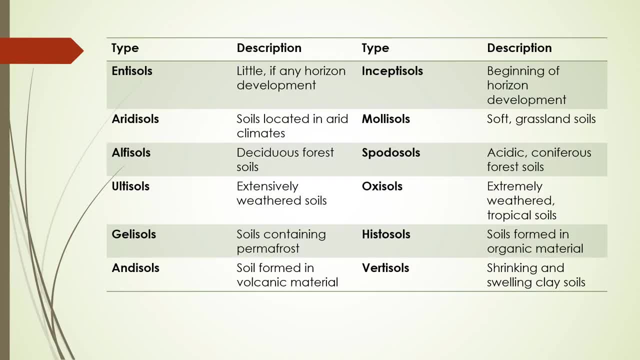 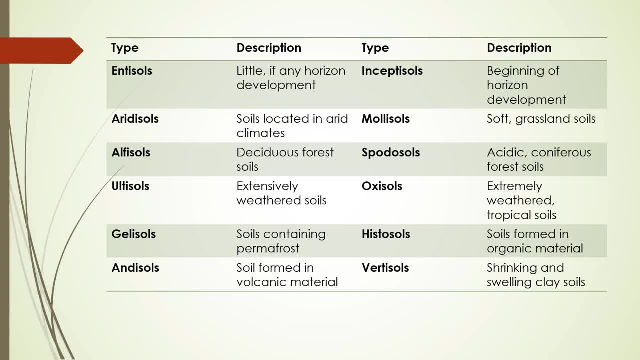 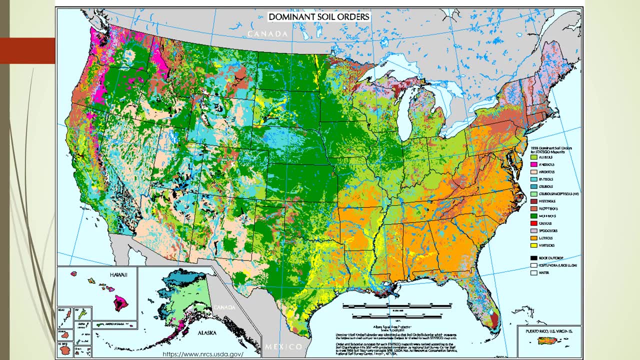 which are formed by volcanic material, and some of these other area are in other areas and I'll talk about each one individually. okay, here are the dominant soil orders and here we've got pink, which is andesols, very fertile, but we'll talk a little bit more about that in a minute. 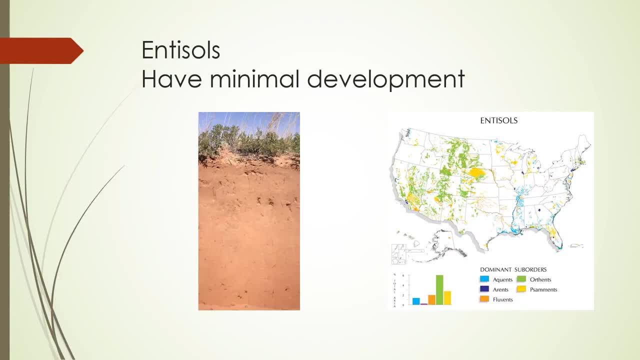 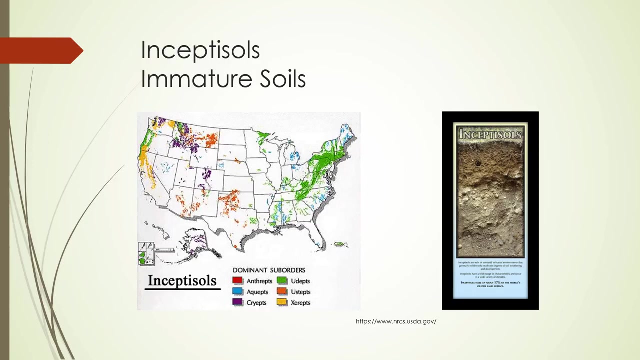 okay. so andesols have minimal development and you can see from this map where you're primarily going to find these areas. very little in our area, quite a bit in the mountain west and the southwest and septa sols are immature soils and we do have some of that you can see in this map here. 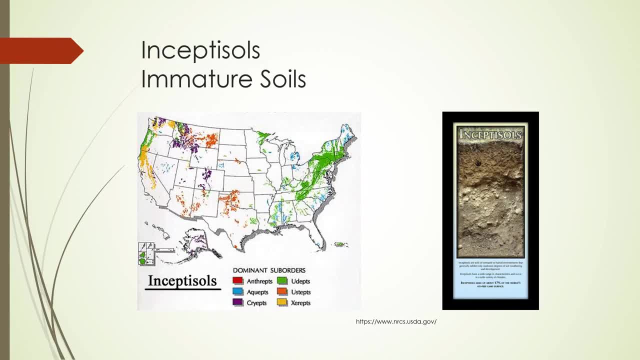 and these are just broken down further into other sub borders. but you can see we have some around the puget sound area because we are fairly new up here, not very well-developed. you can see in the horizon here- it's not a very excuse me- the the yes soil horizons. you can't see a lot of definition between layers. 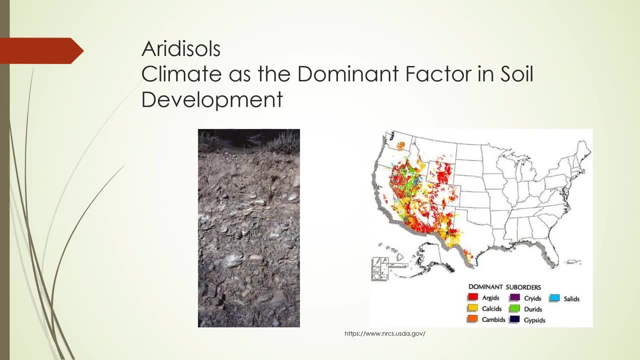 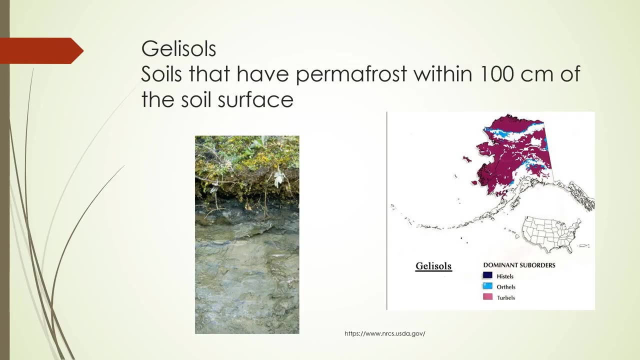 artisols work. this is where climate is a dominant factor in soil development and this is in very arid areas and you can see there really isn't a lot of definition there. we don't have a lot of organic matter, etc. okay, Gelisols are soils that have permafrost within a hundred centimeters of the soil. 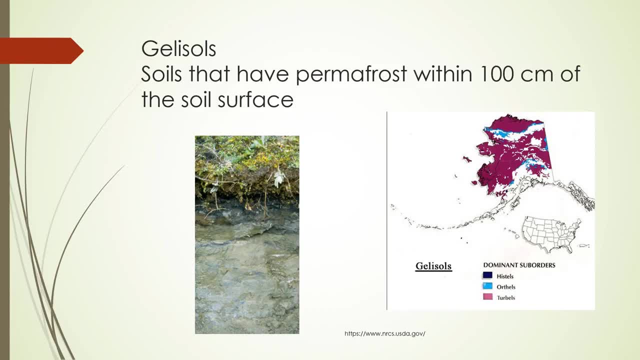 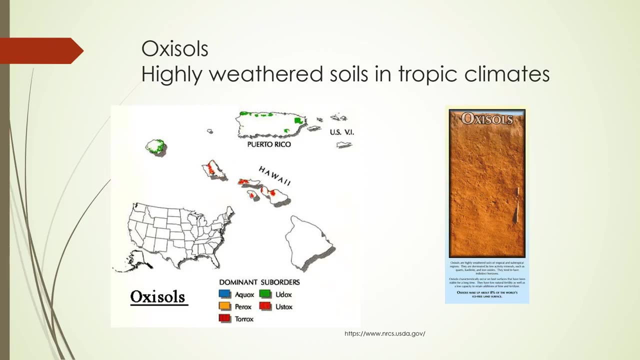 surface and of course that's. you find this in Alaska and not well-defined and very gray in color, so we're not going to have a lot of oxygen in that soil. Oxosols are highly weathered soils in tropic climates- you can see Hawaii, Puerto Rico- and they're very high in iron and aluminum oxides, very acidic. 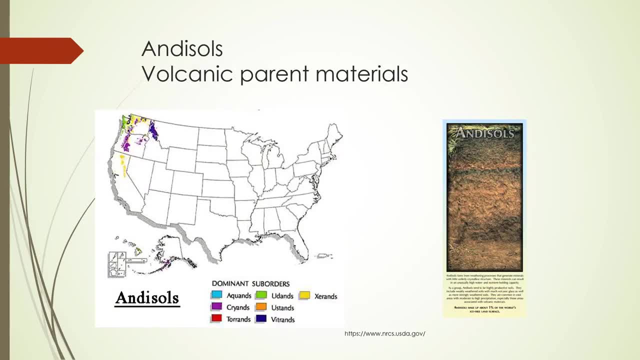 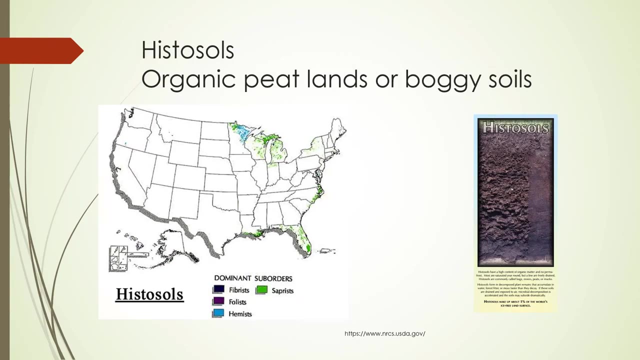 Anisols volcanic parent materials. so we have quite a bit of that in our area, again not super defined, but it's very important to know that. they're very fine in our layers here, but these are very productive soils and very high in natural fertility. histosols are organic peat lands or boggy soils and you can. 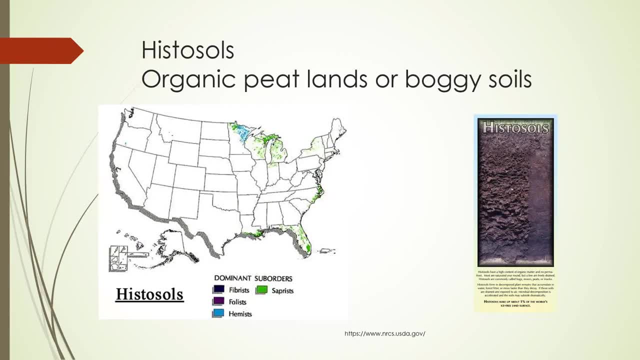 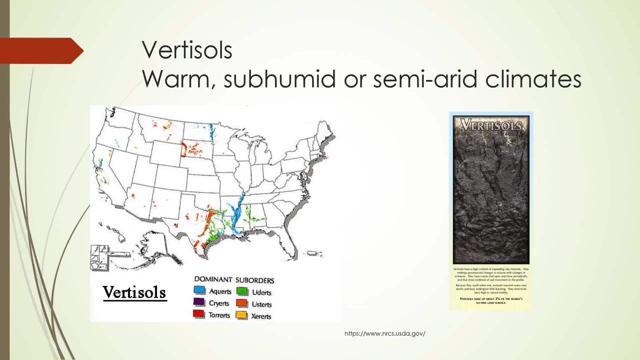 see that's going to be over in the Midwest, in the upper Midwest and some into Florida. vertisols are warm or sub humid. it's warm sediments and they're very high in natural fertility and they're very high in the Midwest and they're very high in natural fertility and they're very high. 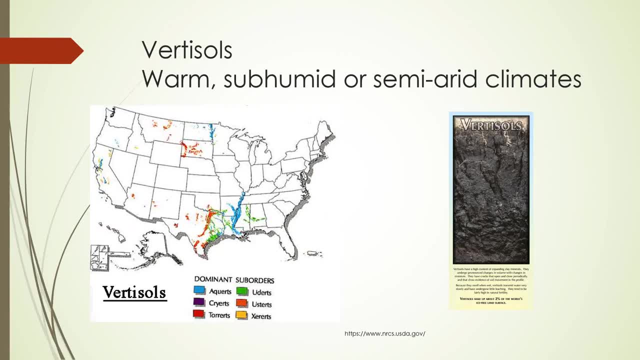 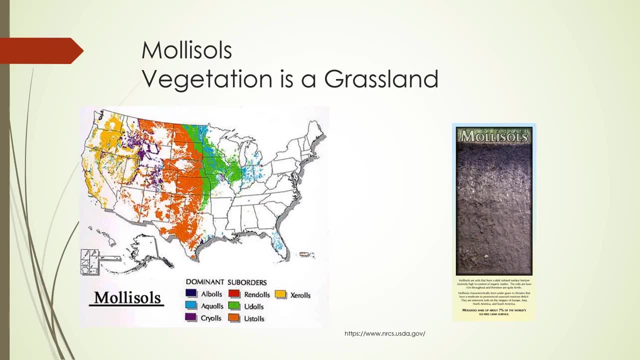 in natural fertility and they're very high in the Midwest. but you can see this is a very subunit or semi-arid climates and that's going to be mostly in the southwest, very dark in color mollusols. vegetation is a grassland, so this is very vertical but fertile excuse. 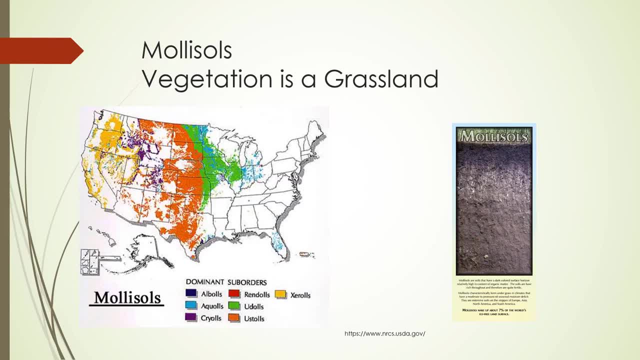 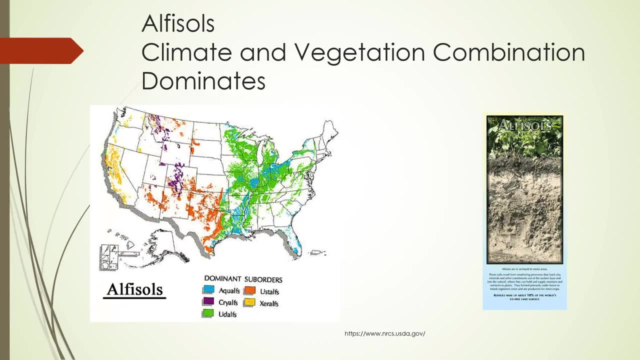 me and probably some of the most fertile soil in the world: very thick, dark colored a horizon rich in organic matter- you can see that here- and vegetation combination- uh, dominations. This is in forest or savanna vegetations, clay in the subsoil, and generally very fertile. 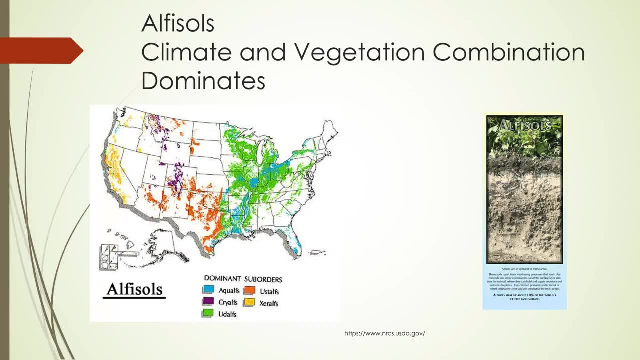 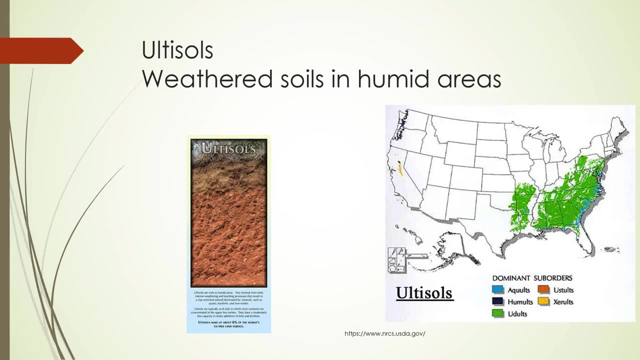 So that's going to be again, uh, near the Mississippi Valley. Utasols. these are weathered soils in highly humid areas and this is going to be, uh, primarily in the southeast, kind of coming up the mid Atlantic coast- um, very low in natural fertility. 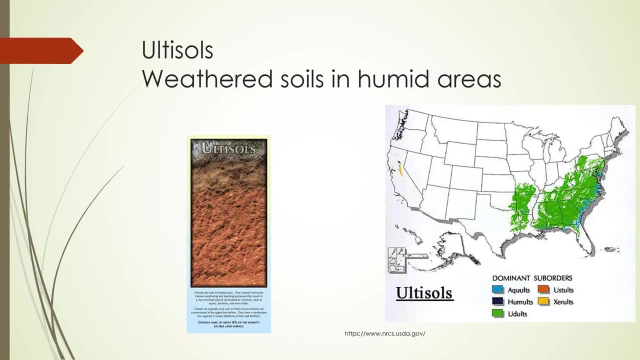 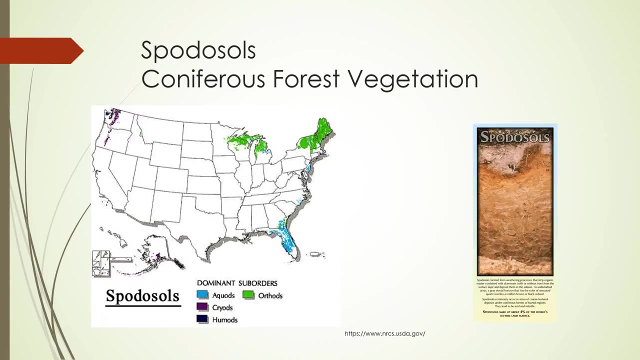 and high in soil acidity. You need to use fertilizer and lime inputs for this to be a productive soil. You can see there's not much in the way of an O layer or a uh a horizon. Spodosols are coniferous forest vegetation. 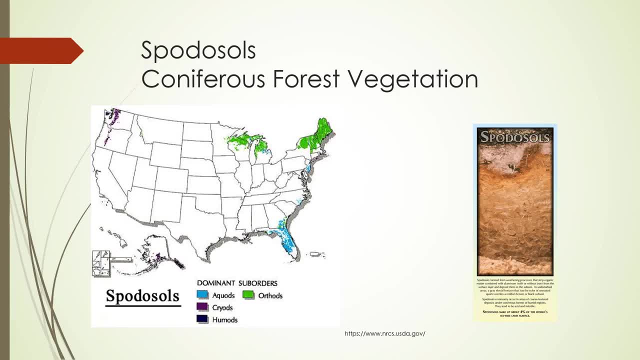 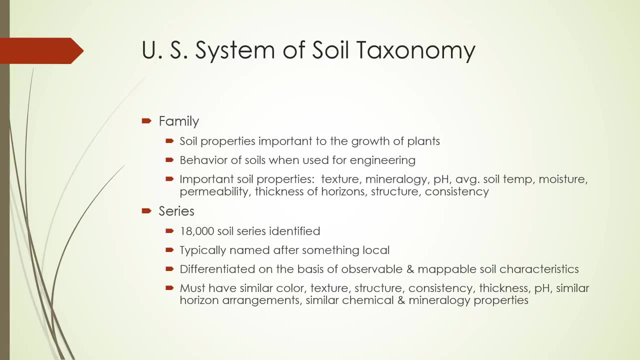 These are our soils in our forest areas: Wet, cool climate, very acidic and low in natural fertility. So we've talked about orders, and then there's family, and family are the soil properties important for the growth of plants. This is also the behavior of soils when used for engineering, and next week we're going. 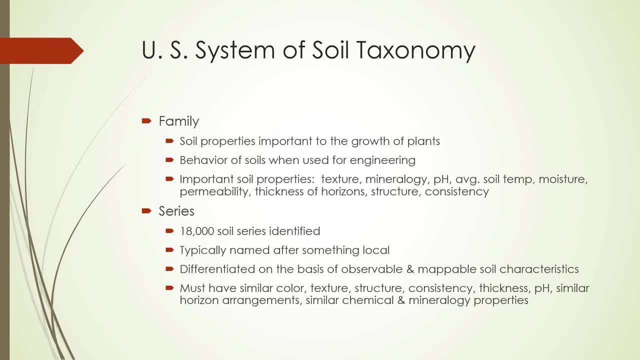 to actually take a look at some soils and uh see if they're useful for uh what we want them to be for. This'll be in a minute. This is in our uh soil survey books. So important soil properties include texture, marine mineralogy, pH, temperature soil. 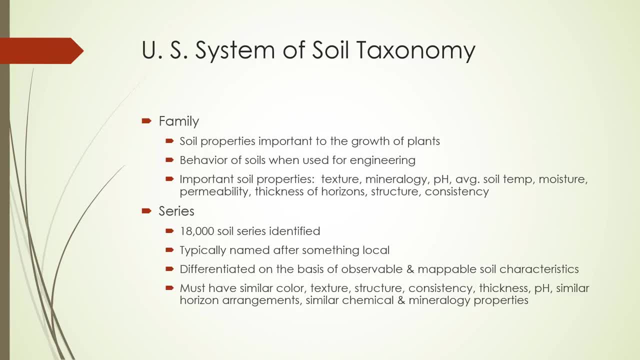 temperature, moisture, et cetera, and then series, which you've probably come across in your studies. uh, of your area, 18,000 soils serve. series are identified. They're typically named after something local. They're different in the basis of observable and mappable soil characteristics. 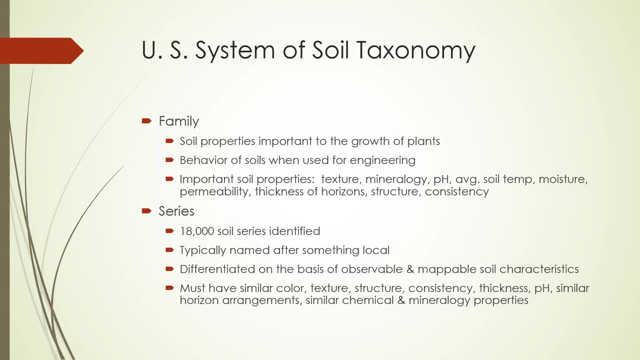 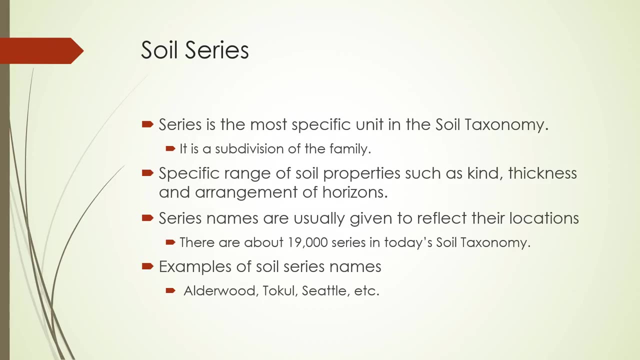 They must have similar characteristics, Similar color, texture, structure, consistency, pH, uh, chemical, chemical and uh mineral, mineralogy, uh properties. So the soil series is the most specific unit in soil taxonomy. It's a subdivision of the family.